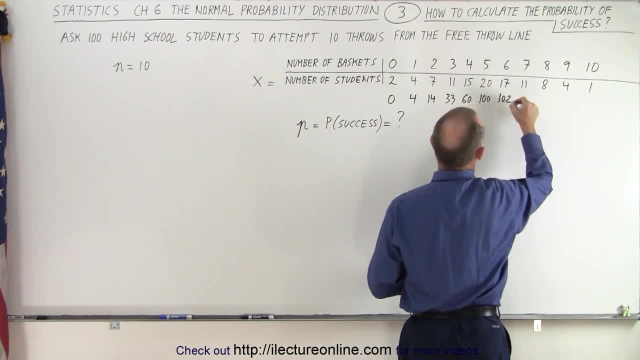 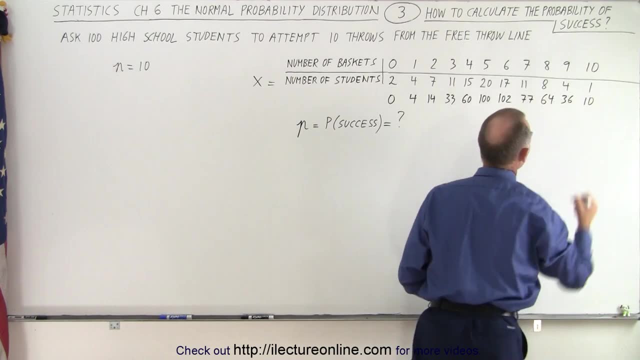 5 is 100.. 6 times 17,, that's 102.. 7 times 11, 77.. 8 times 8, 64.. 4 times 9, 36.. And 1 times 10, 10.. 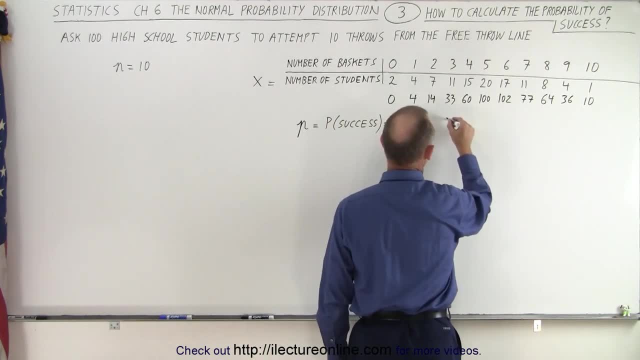 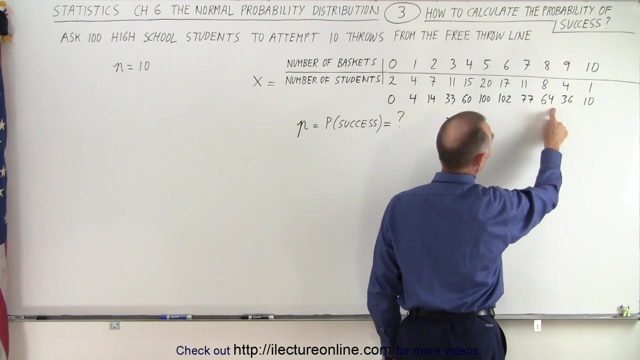 Now we're going to add all those numbers together, So the sum is equal to all. right, that's 18,. that's 21,. that's 51,. that's 111,, 211,, 313,, 320,, 390,, 454,, 484,. 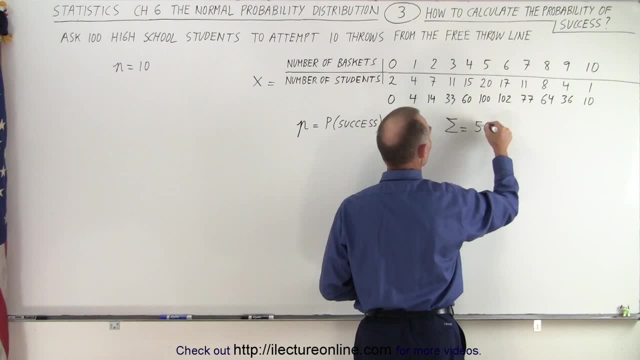 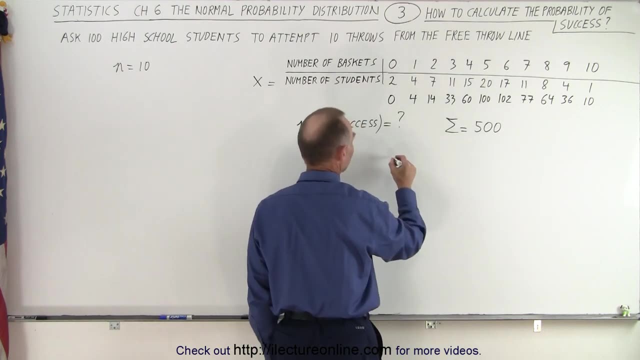 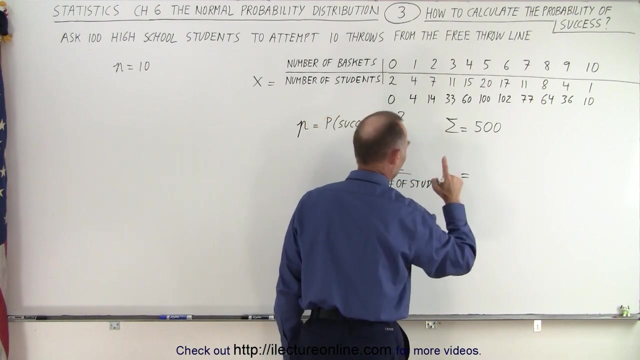 9,500 all together. So the sum of those numbers is 500.. So now that we have those all added together, the next thing we're going to do is we're going to divide the sum by the number of students, And that's going to be equal to 500 divided by 100, which is equal to 5.. Now 5 is. 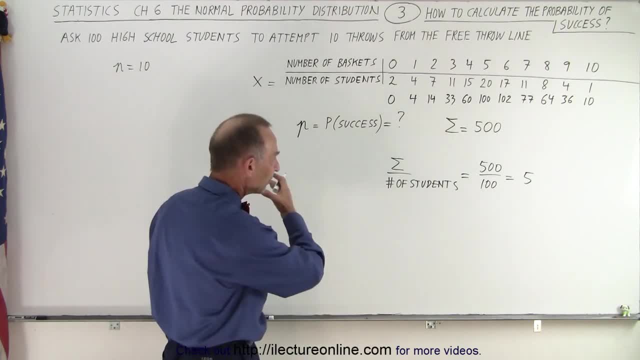 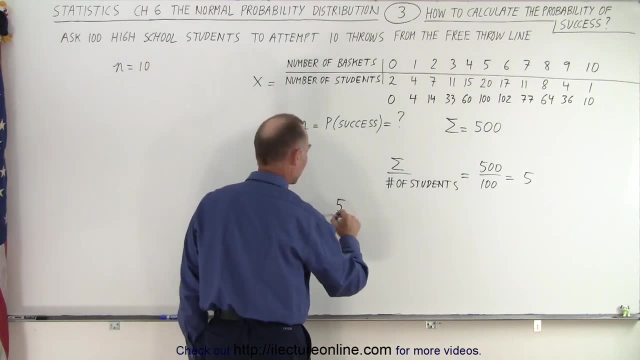 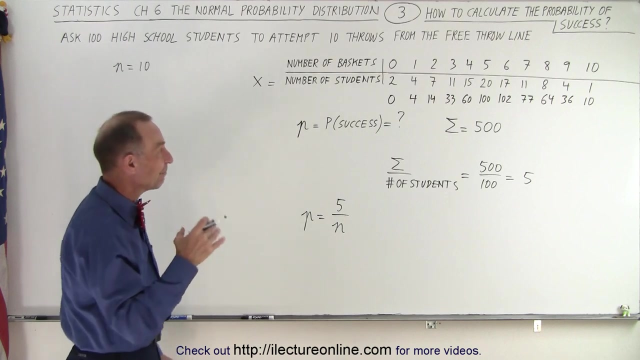 the most probable number of baskets made based upon our calculation. So now to get the probability of success, we take that result- 5, and we divide it by the number of tries. We try 10 baskets and most likely we'll make 5.. So the probability of success, 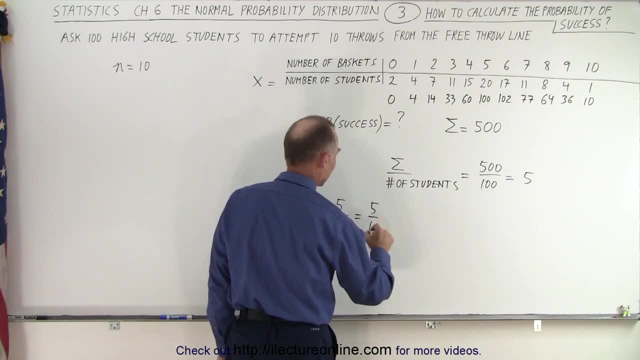 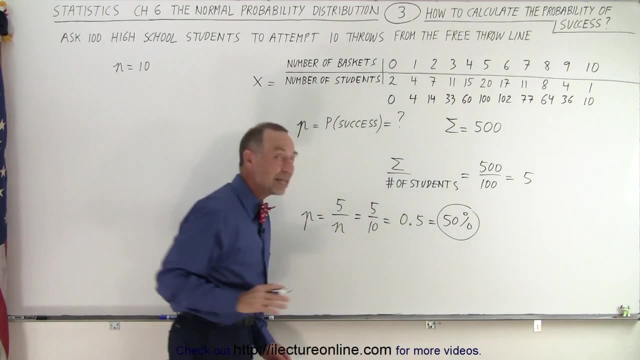 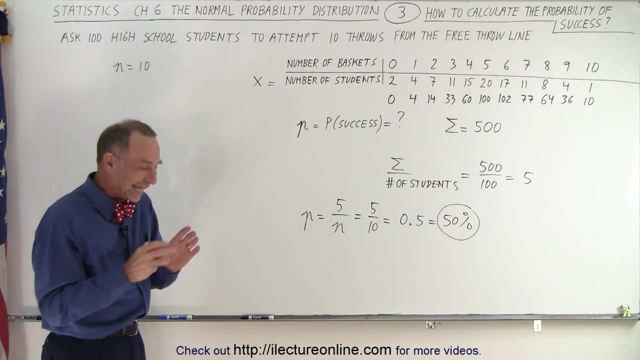 therefore, is equal to 5 divided by 10, which is equal to 0.5,, which is 50%. So what we're saying here is that, with this normal distribution of probabilities, the probability of making a basket at any given time, any one particular student picked. 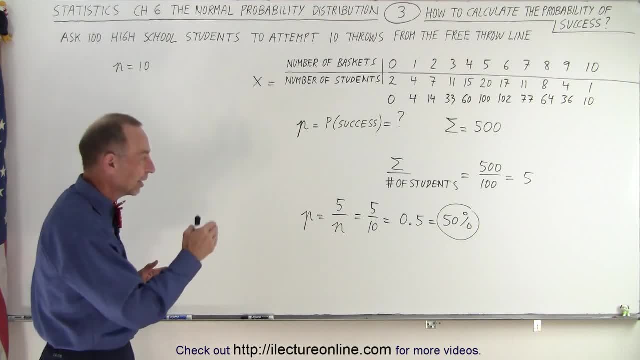 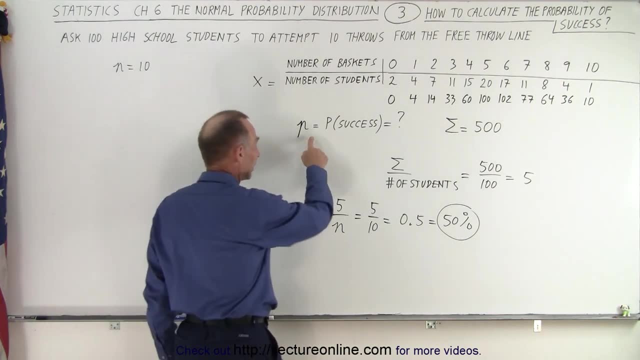 at random and they shoot a basket. the success of shooting a basket is about 50%. They'll make one out of two attempts on average, And so that is what we call the probability of success. Now, why do we need the probability of success? Well, later on we're going to calculate the mean. 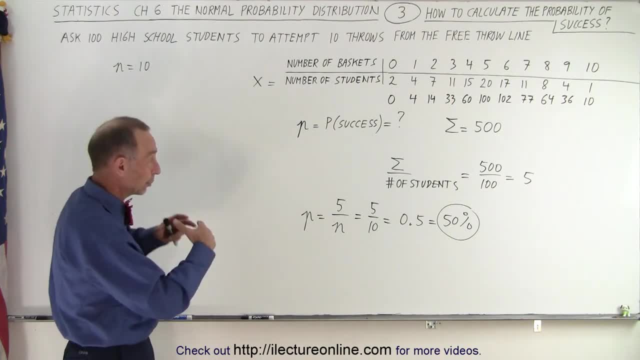 we're going to calculate the standard deviation, And so in order to be able to do that, we need to know the basic principles of how to calculate the probability of success. So we're going to calculate the constituents going into those calculations. So one of them is when we have a 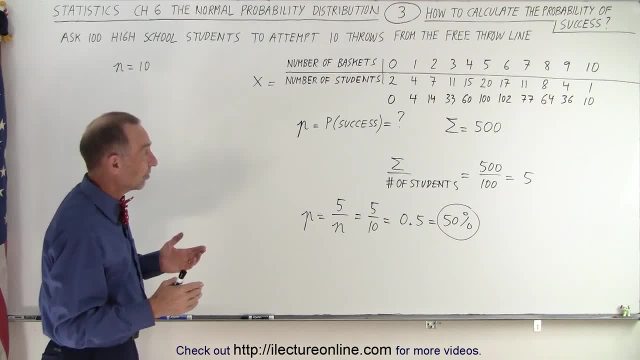 random distribution of events, essentially the random distribution of baskets made. when 100 students are picked and they each are allowed 10 tries, the average probability of success of anyone making a basket at any time is 50%, And we call that the probability of success for this.